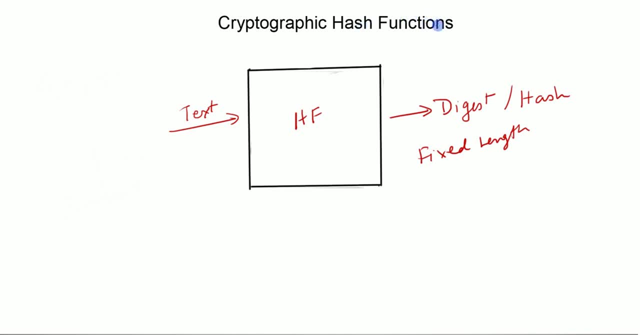 input to its digest, but not vice versa. So it should be very, very hard to actually receive any information from the digest about the input. So let's see how it works. So it's like we cannot get anything out of it, not even its size or whether it's. 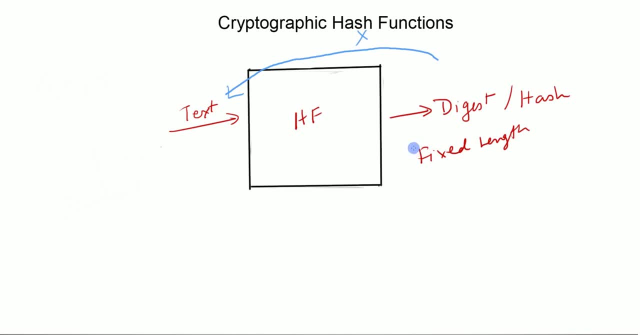 number or text, nothing. Now, I'm not saying that it's impossible. Theoretically it's possible, but certainly it's not feasible practically, because what you have to do is you have to check each and every value that what kind of text or input matches the digest after being hashed. 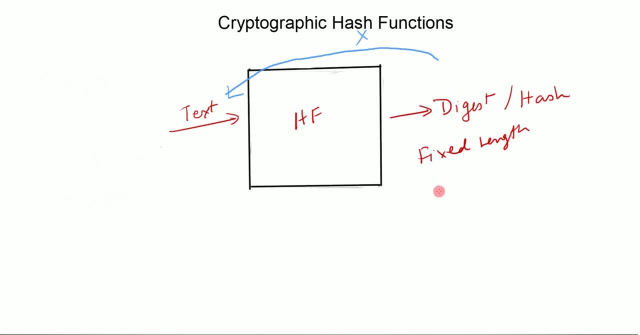 Now the digest after being hashed is a string of fixed length, and what kind of input matches the digest after being hashed? Now the digests should look random. What I mean by this is that if we change a small part in the input text, the whole digest should change. Now I don't mean that as a rule that every character would change. 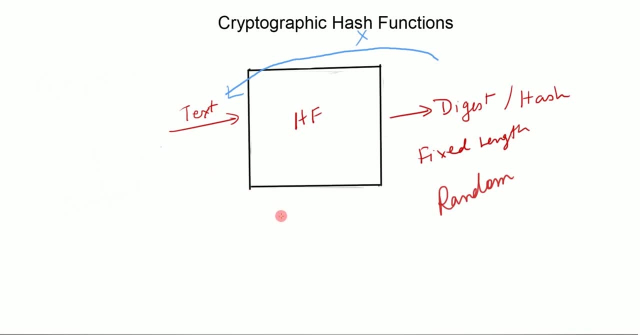 but it should look random, right, Like there should be no pattern between changes in text and changes in the digest. So what I mean by this is, let's say we have a text, hello, and the digest for this is one four, b, e. Now I just have taken a random number and letters This: 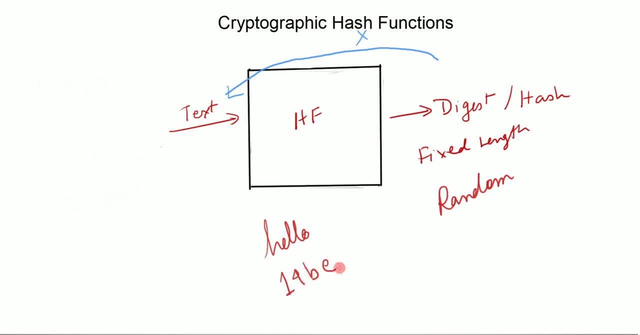 should not be a digest in the real world, because in the real world digests are quite long. So let's say I change the o to p. Now it should not be the case that the b changes to c or it changes with a pattern, The. what should be the case is that 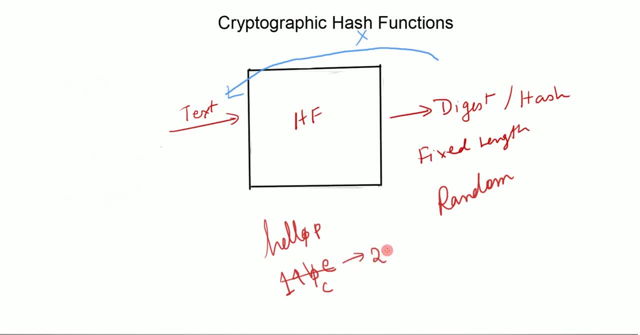 it changes to another completely random value like two, five. let's say a and one. Now, two inputs should not have the same digest. value like t1 should result to d1 and t2 should result to some other d2.. When two values like t1 and t2 end up with the same digest, this thing is called a collision. 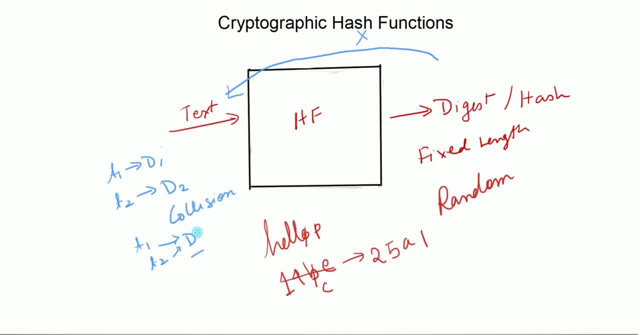 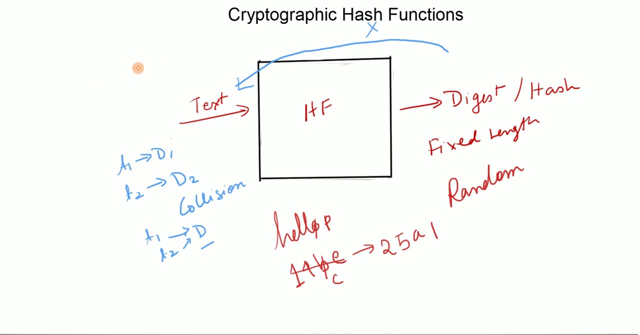 Now our goal is to make our hash functions collision free. Now there are proofs that there may be collisions in hash functions, but finding a duplicate is practically impossible. Last but not the least, the hash functions should not be computationally expensive too much. They should be computationally efficient because we need them in practical applications. Now some 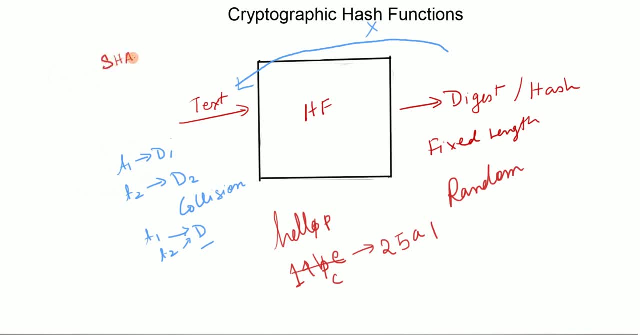 examples of hash functions may be sha256.. It had a precursor, sha1, but it had problems. and there was md4, which is now md5.. I mean, a better version of md4 is md5.. md4 obviously had faults. but there is one thing, guys, that if someone is smart enough, they may come. 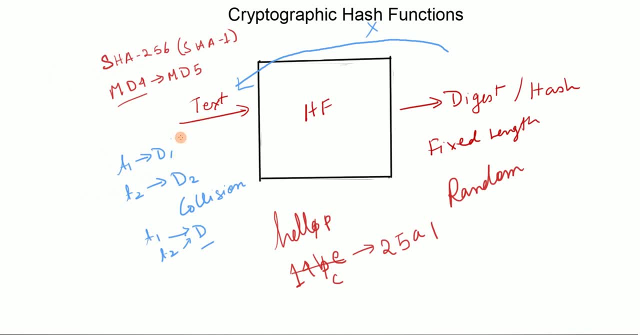 up with a solution to beat these hash functions, There is no guarantee that they won't be ever broken. I am not talking about brute forces. i am talking about if someone is smart enough and they find a cheat so that they can find out the text from the digest without doing a big brute. 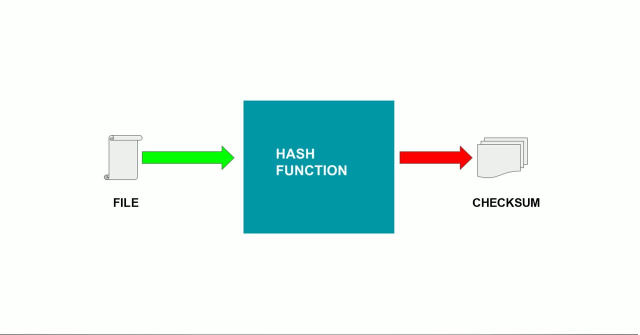 force attack on this thing. There is one more thing that I would like to point out: that not only we can hash some text, but we can have some shutouts on our chit and on ** Jon Wilson��**- I am talking to Ben Lov Paleo. There is one more thing that I would like to point out: that not only we can hash 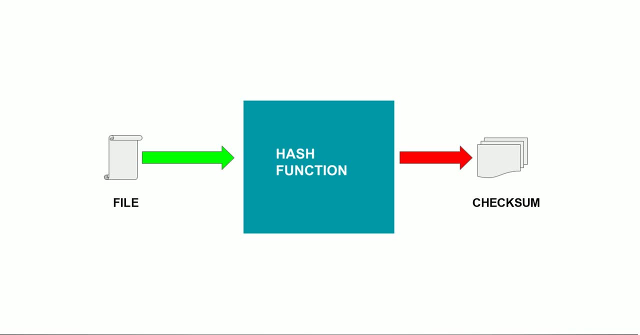 some text, but we can have some shutouts on our chat on these small options. You can find outукаwe text, but we can hash any kind of data. I use text till now in the video for the ease of explaining. In fact, we can hash any file and that has a lot of applications With this. 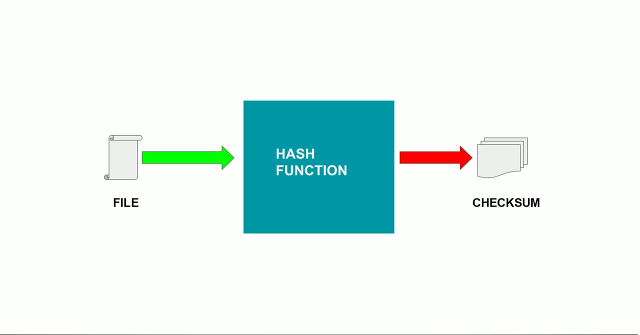 we can track if a file has been changed, Because even if a file has been changed a bit, the hash would change completely. Now you might have seen md5 checksum while downloading a file. Now this is necessarily the md5 hash of the file. Now this is to validate. if the 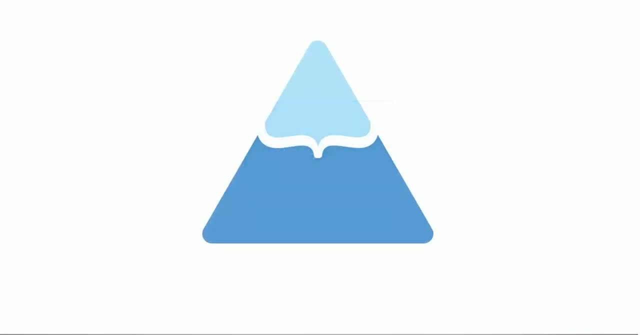 file is corrupt or not. This will be it for today's video. If you learn something new, please leave a like and subscribe to the channel. Put down what videos do you want from this channel in the comments. Guys, stay curious, keep coding and thanks for watching.